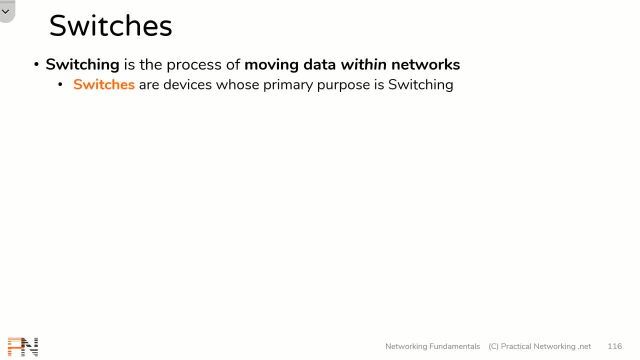 And a switch is simply a device whose primary purpose is switching. We're about to show you an illustration of a switch and everything it does to funnel communication between these hosts, but it's important to understand anything that claims to do switching is going to operate the way we describe a switch to operate. 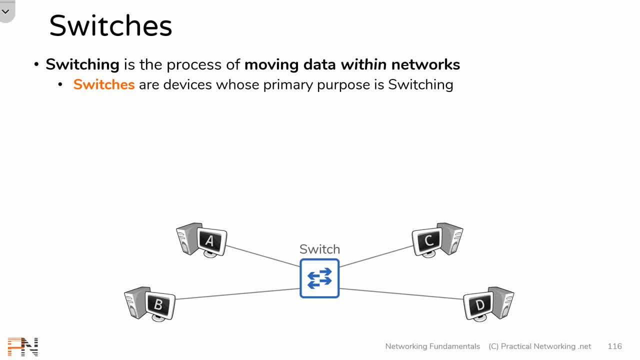 We're simply going to be describing the rules of switching. For these hosts to communicate with one another, they each need IP addresses and MAC addresses. Now, since a switch only facilitates communication within a network, this tells us that all of these devices that are speaking through the switch must belong to the same IP network. 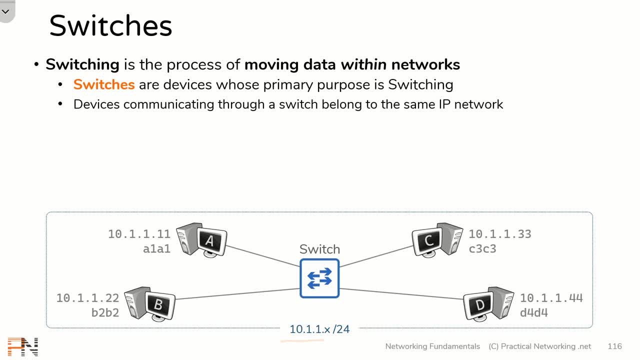 In this case, that IP network is the 10.1.1.x network. In this lesson we're going to illustrate everything that the switch does to enable communication between host A and host D. Now, in the last lesson we described the host role in all this. 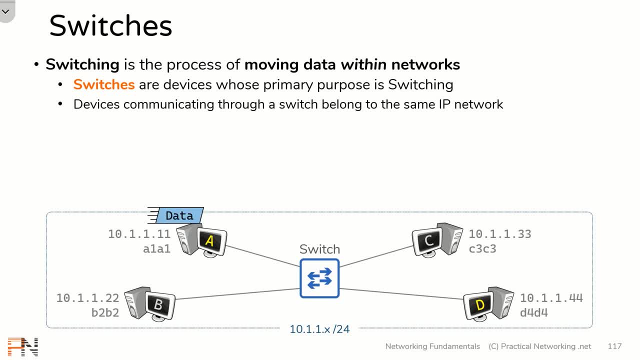 We described that the host is going to generate some data to send to host D and then add a layer three header to that data which includes the source of host A and a destination of host D's IP address. Then host A is going to perform ARP to figure out the MAC address which correlates to that. 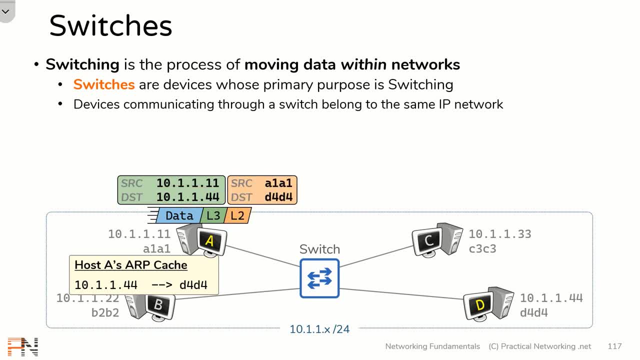 destination IP address. Then host A is going to add a layer two header which indicates host A's IP address. Then host A is going to perform ARP to figure out the MAC address which correlates to that destination IP address. Then host A's MAC address and host D's MAC address. 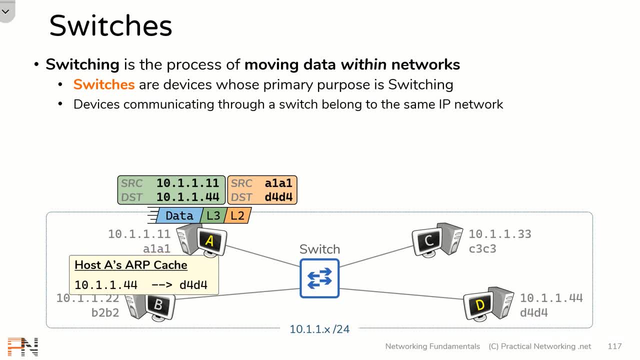 All of that we described in the last lesson and all of that still applies In this lesson. we're just going to be focusing on the switch. If you recall, a switch is a layer two device, which means they're only going to be using. 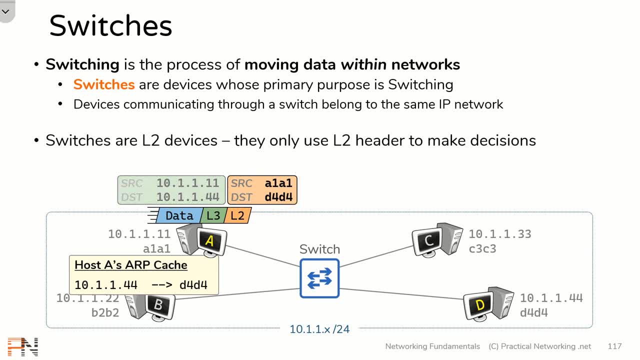 the layer two header to make their decisions, which means the switch doesn't look at the layer three header at all. In fact, everything after the layer two header from the perspective of the switch is simply considered data. You and I know there's a layer three header in here. 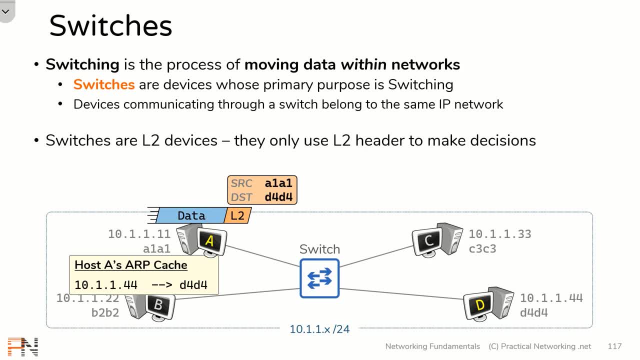 But from the switch's perspective, it doesn't care about that layer three header, It's just going to make its decision based upon the layer two header. In fact, we can actually get rid of anything IP related on this topology, because if all, 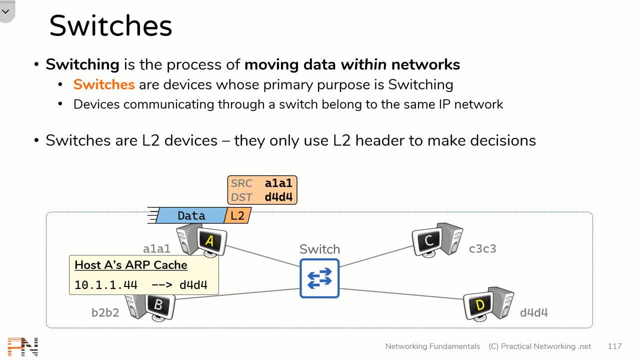 we're doing is focusing on the switch. we don't actually need to consider the IP addresses that are communicating. We're going to show you everything that happens to get this data to host D through this switch. Now I want to point out that we are starting from the position that host A already knows. 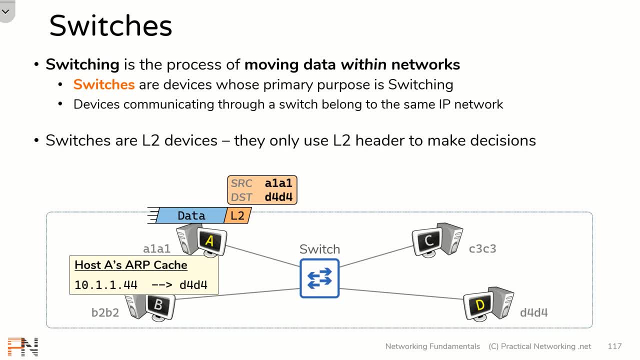 the MAC address it's trying to speak to. Normally, host A would have to discover the MAC address that host D is trying to speak to. We can do this using ARP, but for our illustration we're going to assume host A already knows. 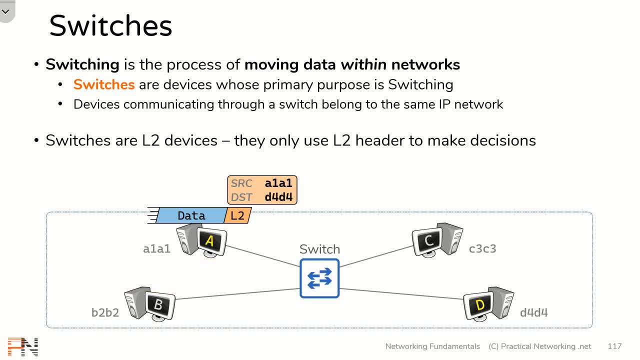 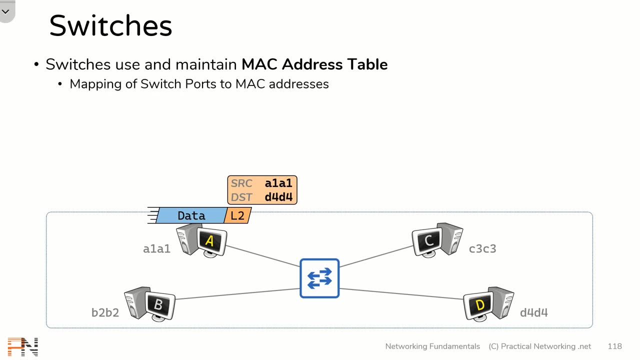 the MAC address it's trying to speak to, so we can leave ARP out of this illustration entirely. With that said, let's go ahead and explain how switches facilitate communication within networks. Switches use and maintain a MAC address table. A MAC address table is a mapping of switch ports to MAC addresses. 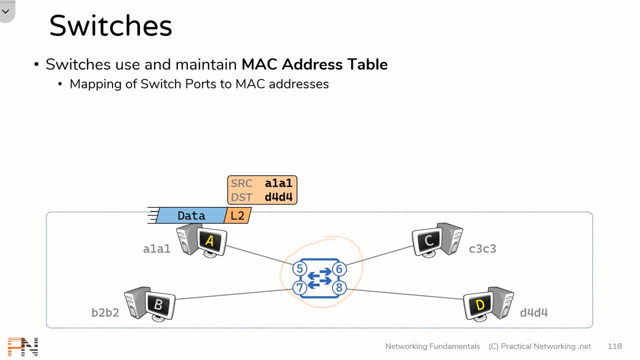 Each of the hosts in our topology are plugged into this switch in a particular port. For instance, host C is plugged into port six. Now every different switch out there uses different numbering schemes for their ports. For the sake of illustrations I'm just going to use these numbers: five, six, seven and. 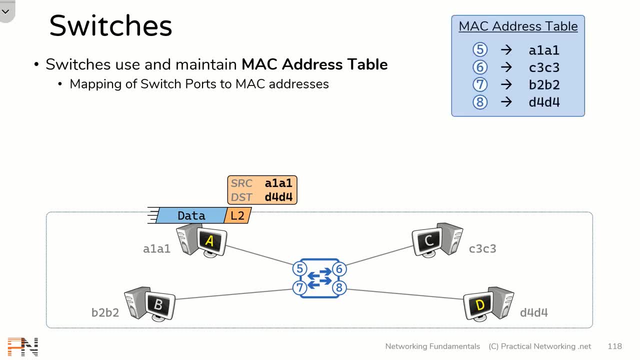 eight. A MAC address table, then, is going to include the mapping of a particular switch port and the device that's connected to that port, meaning it's going to know that out port seven exists a device with the MAC address B2B2.. 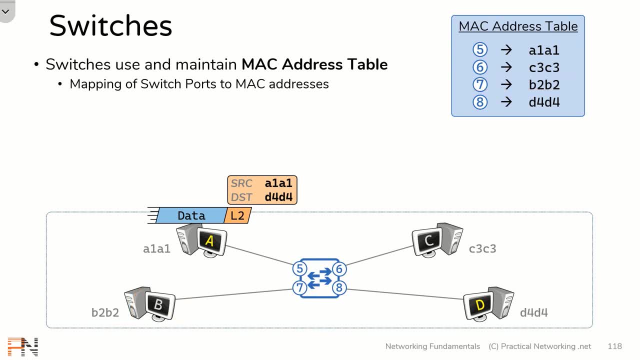 Now this MAC address table doesn't start out populated. In fact, it starts out empty and as data is flowing through this topology, the switch will populate this MAC address table. So let's look at the MAC address table. Beyond this MAC address table, the switch is only ever going to perform three actions. 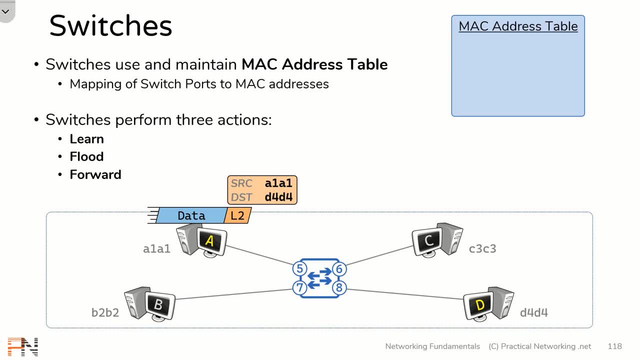 Learning, flooding and forwarding. If you understand these three actions, then you'll understand how switching works. Every switch you come across, regardless of the platform, regardless of the vendor, regardless of the code version, is only going to do three actions. 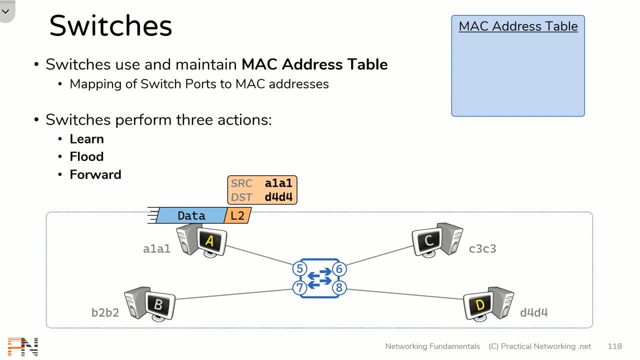 These are actually the rules of switching in general, So let me show you how they work. So host A is going to start. Let's start by putting this information on the wire That will arrive on the switch on port five, and this is going to allow the switch to perform. 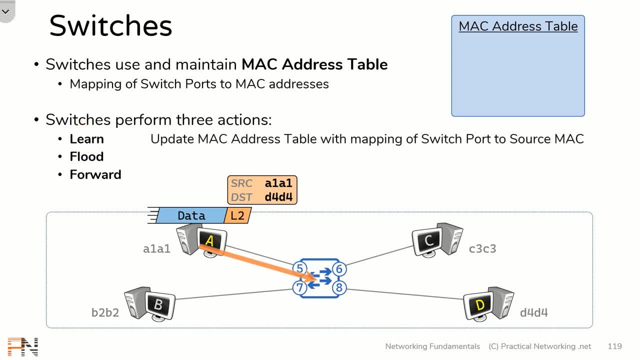 its first action, which is to learn, The learning action has the switch update its MAC address table with a mapping of the switch port and the source MAC address of the received frame. meaning on port five. this switch just received a frame with a source MAC address of A1A1, which allows the switch. 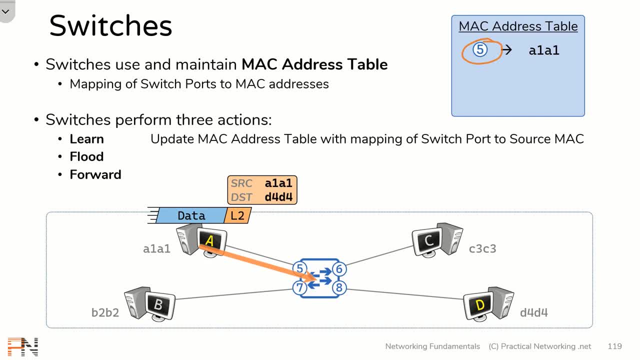 to update its MAC address table. Okay, So the device on port five owns the MAC address A1A1.. That is the learning action and the switch is going to try to learn the source MAC address for every frame the switch receives. Now the switch has to figure out what it's going to do with this frame. 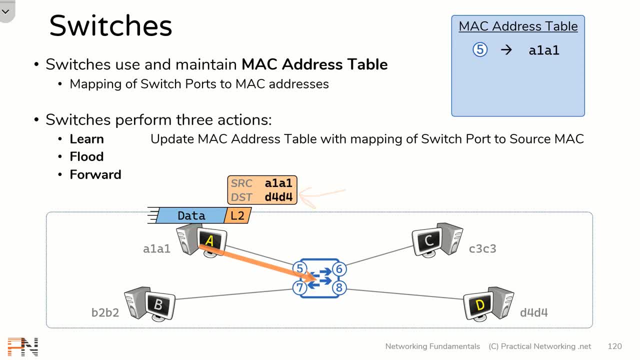 It's going to look at the destination address of that frame to determine that this is meant to be delivered to the device that has the MAC address D4D4.. You and I know that that device exists over here. Okay, The switch will list everything that the switch knows. so at this point in time, the switch 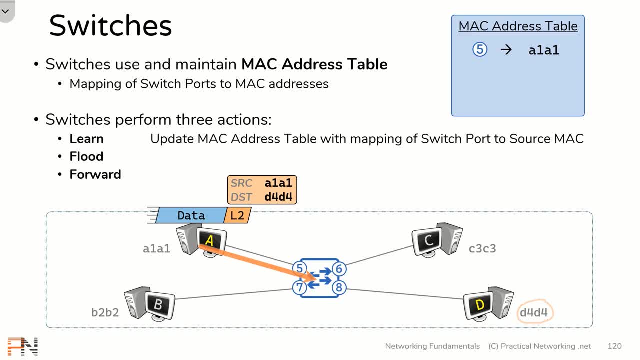 does not know what port the MAC address D4D4 exists out of, which means the switch's only option is to duplicate that frame and send it out all ports. This is the only way the switch can ensure that whatever owns that MAC address does get. 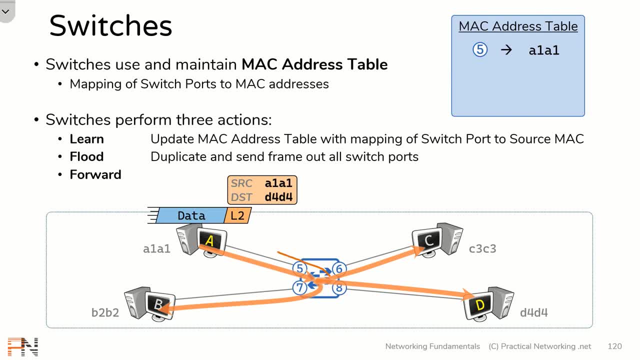 this frame. Now notice that the switch did not forward the frame back out port five. When it duplicates the frame and sends it out all ports, it's going to send it out all ports except the port that received the frame initially. The idea there is that if this frame arrived on port five, there's a good chance that the 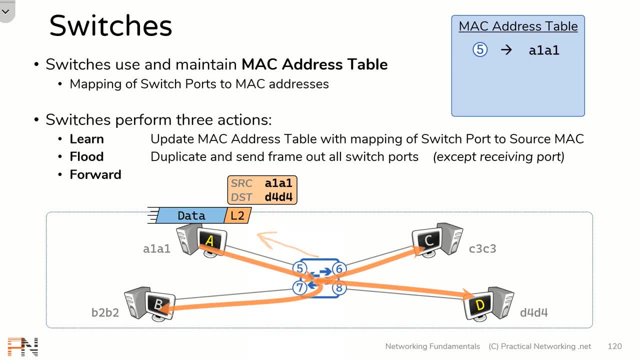 destination does not exist back out port five. So that is the flooding action and all other hosts in this network are going to receive a copy of this frame And when host B and host C receive this frame, they're going to look at the destination MAC. 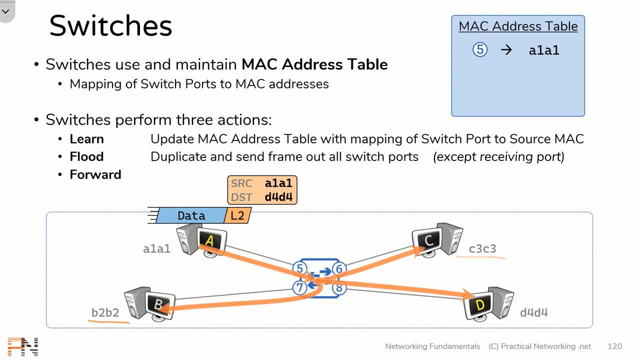 address to determine that they are not the intended recipient for that frame. They are therefore simply going to silently discard that frame. Okay, Host D, however, will be looking at the destination MAC address to realize it is destined to host D and host D will accept that frame for processing. 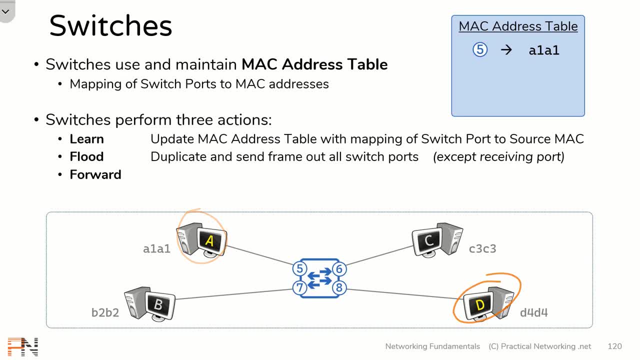 And that is how data will get from host A to host D. Now, inevitably, host D is going to generate a response to send back to host A. This response is going to have a source MAC address of host D's MAC address and a destination MAC address. 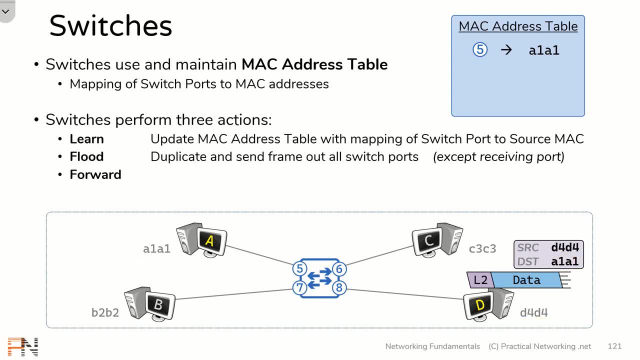 of host A's MAC address. Host D is going to put this response on the wire, where it'll arrive on the switch on port eight. This will allow the switch to once again perform its learning action. It's going to update its MAC address table, indicating that something just arrived on. 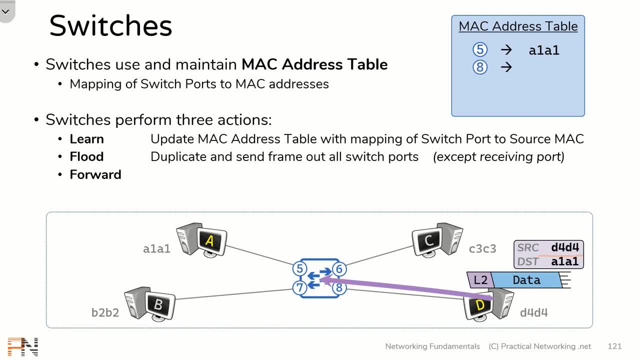 port eight with a source MAC address of D4, D4. This allows the switch to create this mapping. Now the switch is going to try and figure out what it's going to do with this frame And once again it's going to look at the destination MAC address, A1, A1, to determine. 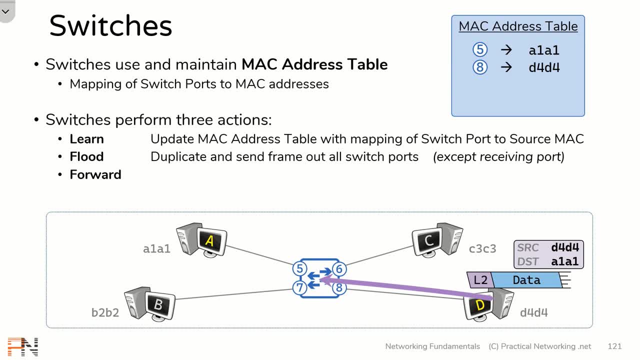 where to send this frame next. The difference, however, is that now the switch knows how to deliver a message to host A1, A1. It knows how to deliver a frame to A1, A1.. It knows that A1, A1 exists out port five. 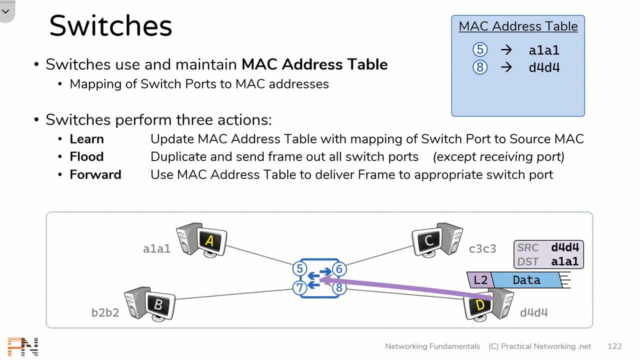 This will allow the switch to simply forward that frame out the appropriate switch port. That is the third action of the switch, the forwarding action. The forwarding action allows the switch to deliver a frame directly to the appropriate switch port because the destination MAC address exists in the MAC address table. 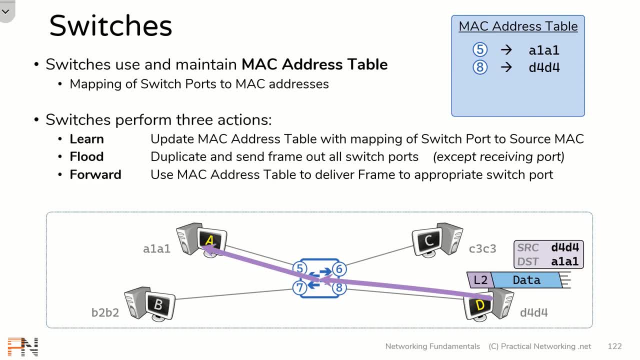 This will allow the switch to send that frame directly to host A, And that is how the response is going to be generated, And that is how the response data will go from host D to host A. Now, at this point, anything else that A and D need to send to each other will simply go. 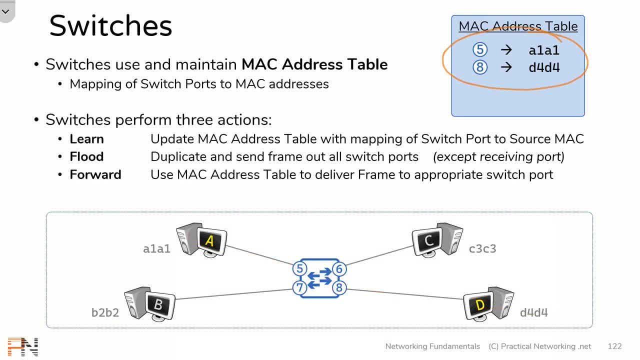 directly to each other. Now that the MAC address table is populated with either of those hosts' MAC address, anything A and D send to each other is going to go directly to each other without having to do the flooding action, which means host C and host B will not get a copy of any of. 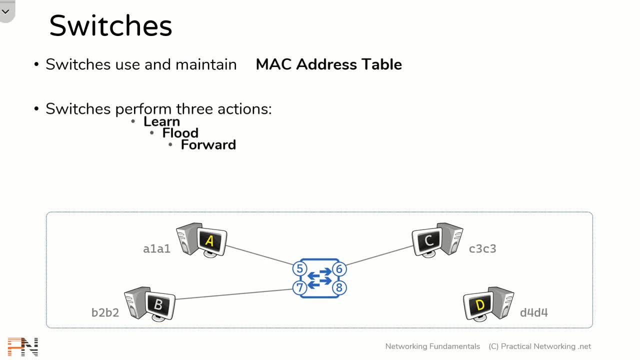 that data. And that wraps up our discussion of how switches work. Again, switches use and maintain a MAC address table, which is a mapping of a switch port to a MAC address, and switches perform only these three actions. If you understand these three actions, you now understand how any switch for any vendor. 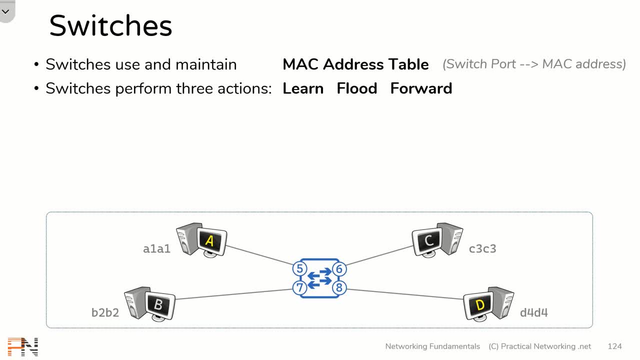 on any platform facilitates communication within a network. But before I let you go, there are two more ideas. I want to leave you with Our illustration. involved: host A sending a packet to another host, But everything else is a process. Everything we just showed you would still apply if this wasn't actually a host. and 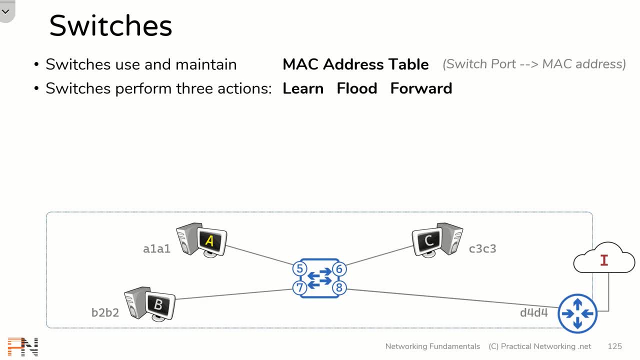 it was instead a router and host A was trying to send something to the router in order to speak to something else out on the internet. The only thing that would be different would be the layer 3 header And, as we discussed, the switch doesn't even look at the layer 3 header to do its job. 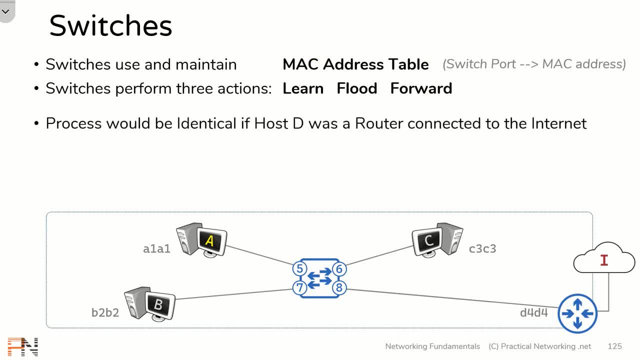 Which means this process is exactly the same whether host A is speaking to a host on the local network or trying to send something to a router in order to speak to something on a foreign network. The second idea I want to leave you with is that we showed you how traffic flows through. 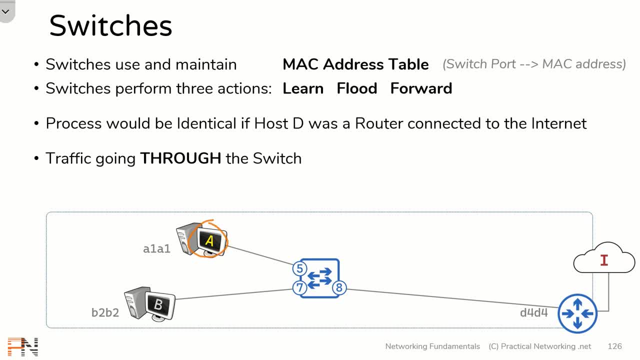 the switch. We illustrated host A sending something through the switch initially to host D. Understand that switches have MAC addresses. Again, any NIC has a MAC address, But you'll notice that this MAC address was completely uninvolved for any communication going through the switch. 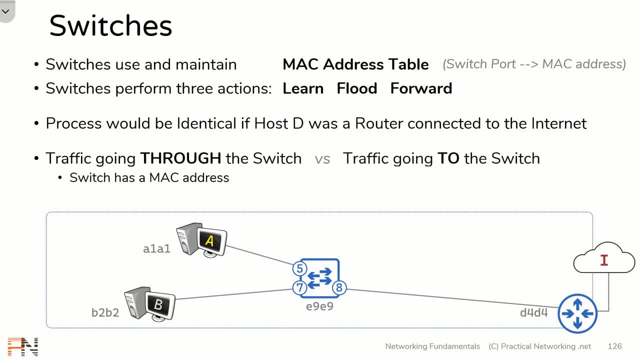 But what if you wanted to send something to the switch? Well, if you're trying to send something to the switch, you'll need to send something to the switch, And if you're trying to send something to the switch, then this MAC address would be: 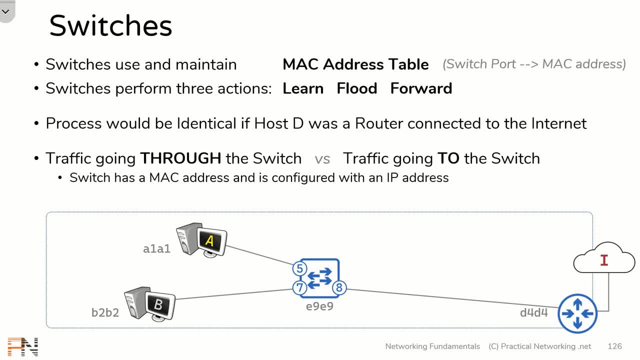 involved. But not only would the switch need a MAC address, it would also need an IP address. And at this point, if you've configured an IP address on the switch and you're trying to send traffic to the switch, the switch is essentially acting as a host on the local. 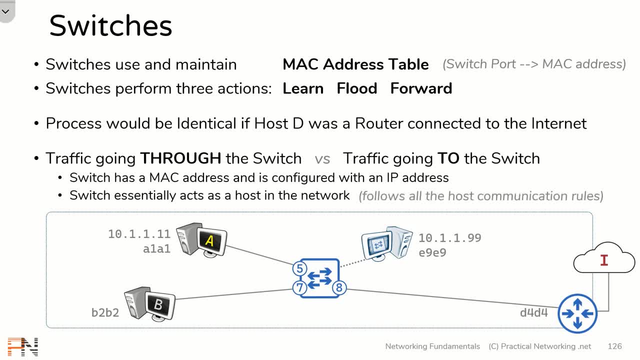 network. It's going to follow all the rules that we described in the prior lessons that hosts follow in order to communicate on a network. The switch's MAC address and also its IP address will also be involved, And if you're trying to send something to the switch, then this MAC address would be. 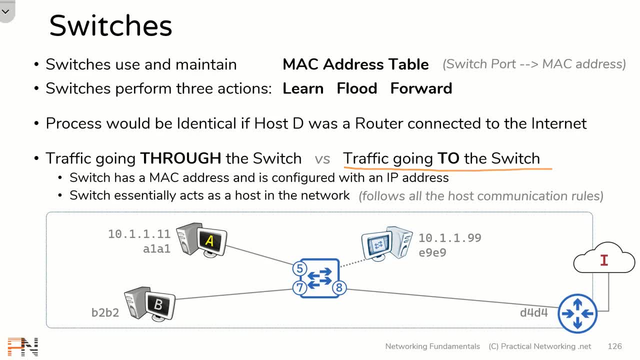 involved. So the switch will only be used if you're sending traffic to or receiving traffic from the switch And if you're trying to log into the switch using telnet or ssh in order to manage the switch. But for any traffic going through the switch, the switch MAC address and IP address will. 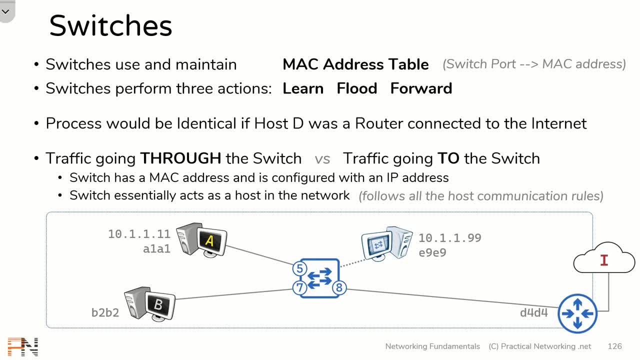 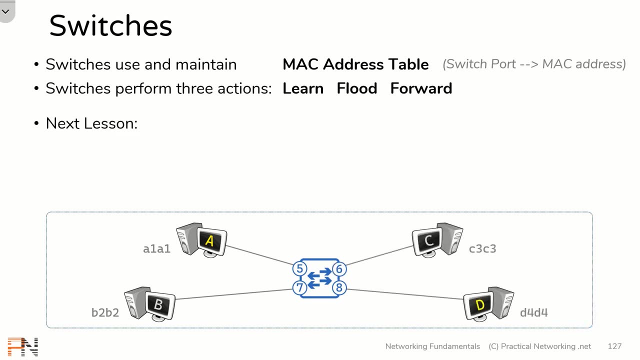 be completely uninvolved in the process. The switch is merely going to perform these actions over here in order to facilitate communication within a network, And that one of our lesson on switches. In the next lesson we're going to unpack three more ideas.